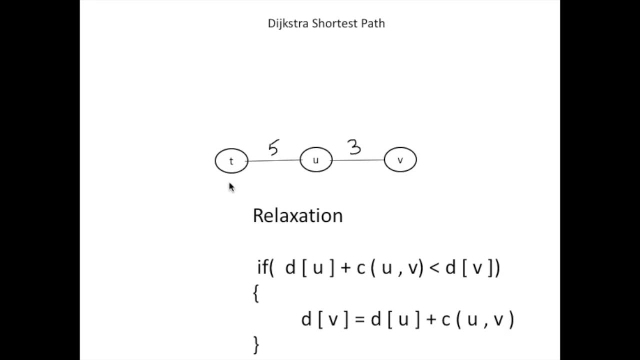 via other vertices, about a procedure, how to find the shortest path. for that. we look at a condition that is a relaxation condition. so here i'll show you. let us find the distance for each vertex, as this is our starting vertex, so distance for this vertex is zero. and from the starting vertex to u 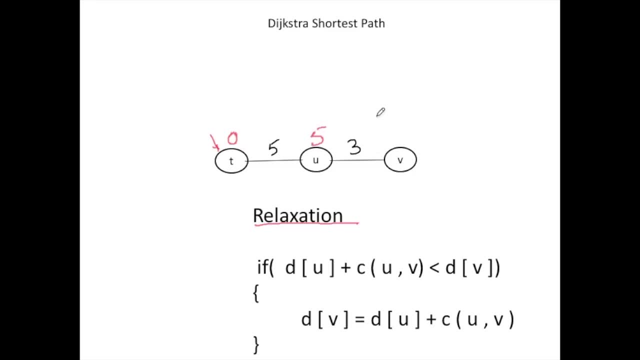 the distance is five and from t to v there is no direct edge. so i say this is infinity. so if i stop here, i can say that the shortest path from t to u is 5 and t to v is infinity. i can stop here. but now, if i follow the extra algorithm for finding the shortest path, containing 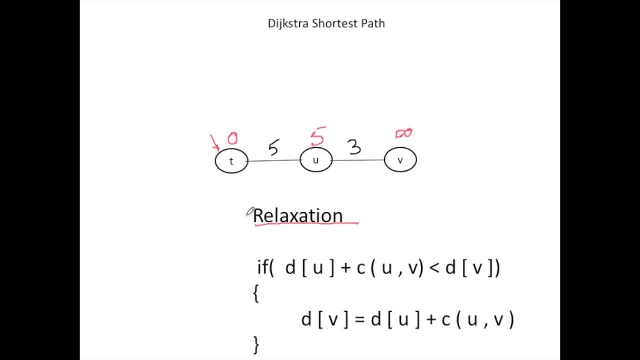 one edge or more than one edges also. so here i check this condition and try to update the vertices. if i say there is a shortest path from t to u that is of distance 5, and if i select this, once i select this, i see that vertex u is then a shortest path to any other vertex. so i will check this condition. 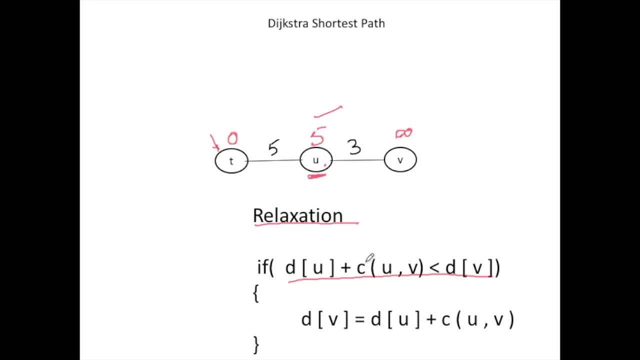 check this condition. the distance of u plus cost of an edge u to v, that is 5 plus 3, that makes 8 and that is less than distance of v. yes, this is infinity. so update this one: distance of v, make it as 8. so this what this vertex is relaxed. 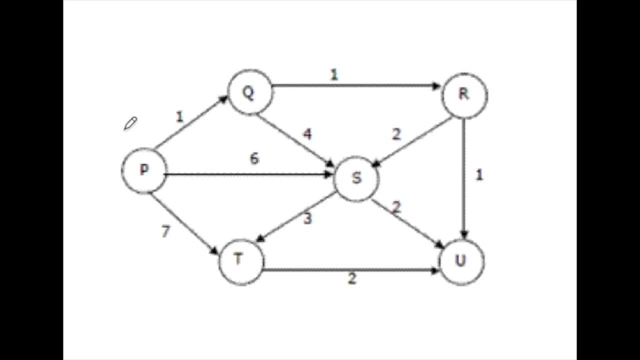 so, after checking this condition, see how the extra algorithm works. if i make this as a starting vertex and the distance of this vertex is zero and distance from p to q is one and p to t is seven, p to s is six and p to r, there is no direct edge, so let us make it infinity. 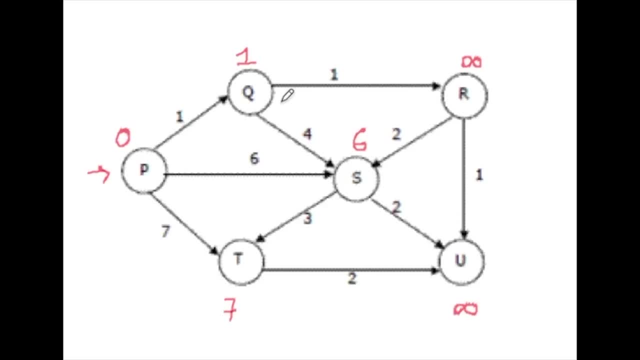 edge. So let us make infinity. Now I have labeled all the vertices and found the distances from the starting vertex to that particular vertex. Now I have to find the shortest path to all the vertices. So here I start the procedure. I have to pick up the shortest path. 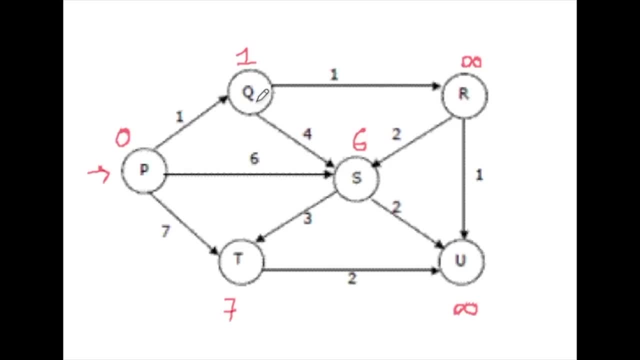 first Means from P which vertex is closest or very much closer to P. So that is Q. So I will select this vertex. Once I have selected this vertex, I have to see that are there any vertices that are going to get relaxed? So yes, see this one, One plus one that 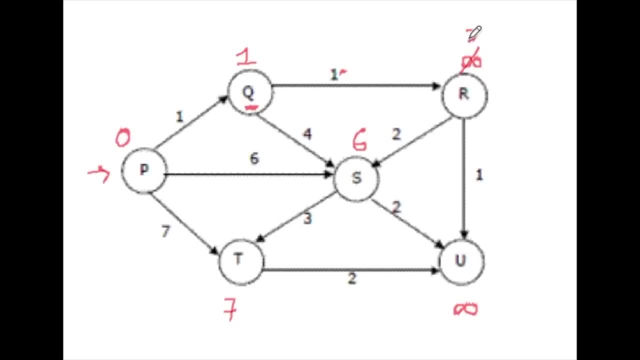 is two. So this is infinity. Now change: We got a shorter path from Q to R. that is two. So the total path from P to Q and Q to R, the cost is two. And next, here it is. 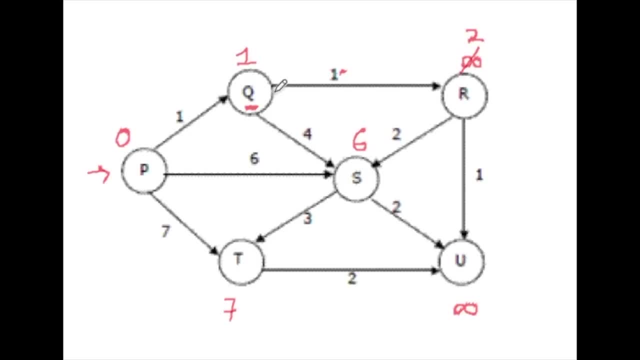 one plus four, But right now it is labeled as six. So one plus four is five, So this is shorter than the existing path. Then, from Q, there are only two edges. Leave it Now, as we have selected Q. Now we have to select the next shortest path. So the remaining vertices: 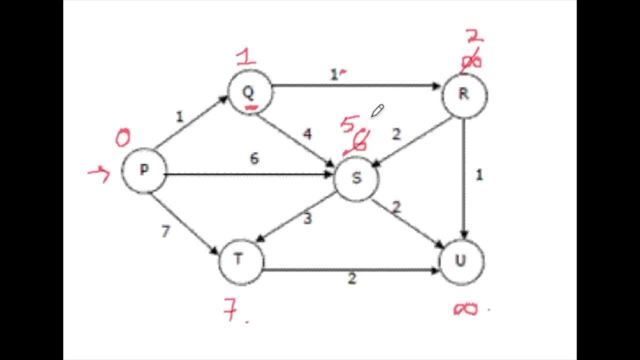 for which we have the paths are seven, infinity, five and two, So this is shortest one, So I will select this one. This is the second vertex I am selecting From here. I will see. are there any vertices? who are having shortest path via R? Yes, two plus one, that is three, So this is infinity. 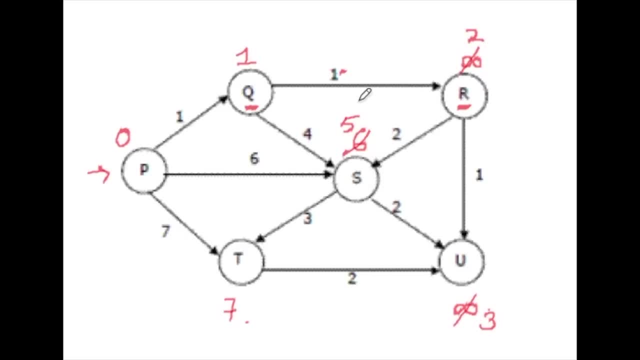 Change it to three And two plus two. that is four, So right now it is five. So this four is smaller than that, So I will take four. So these are two vertices are updated. Yes, Now how many vertices are remaining? T, N, U and Z. 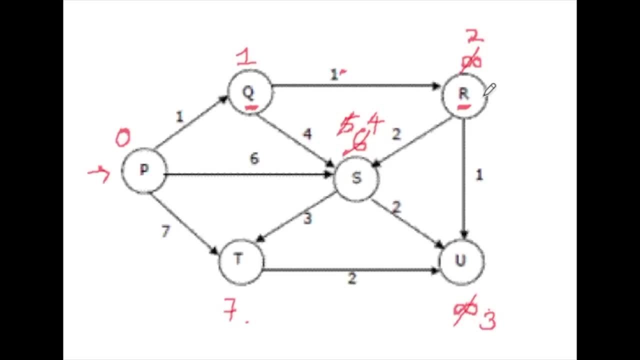 Yes And S3 are remaining. Two are already selected. We found the shortest path. Now I have to pick up the next smallest one. The next shortest path is U, That is, the distance is three. So from here I should check. is there any update to other vertices? Is there any shorter? 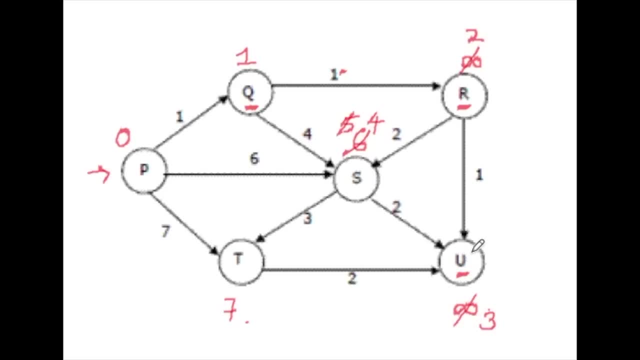 path to other vertices from U. So from U. there are no edges going out, So I will just leave it. Now I have to find a shorter path. next one, That is: this is four, So I will. 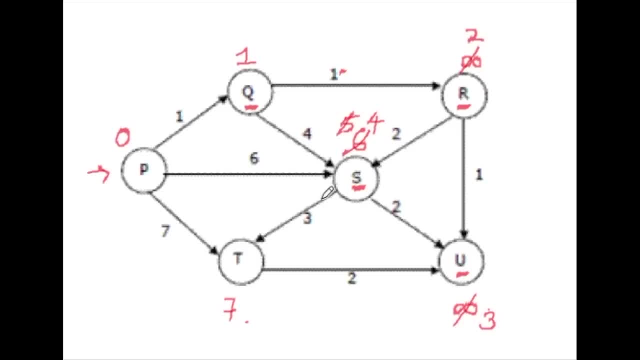 select this one. This is the shortest one. Next, four plus three is seven. This is already seven, So there is no change. So that's all. S is also selected. Now. the only vertex that is remaining is T, So I select that one also. 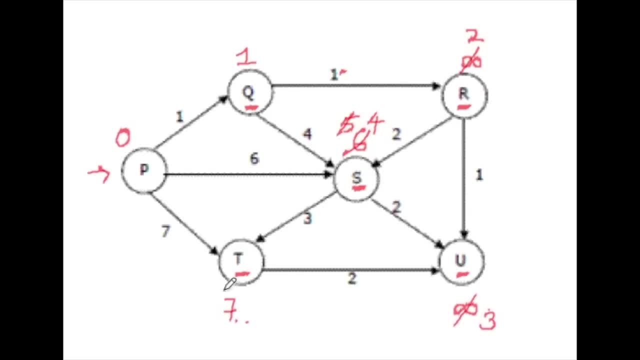 So the cost of the path is still seven, Right. So now, here you can see that all the vertices are labeled with their shortest paths. So from P to Q, it is one, From P to R, it is two. So that is coming via Q, Then P to 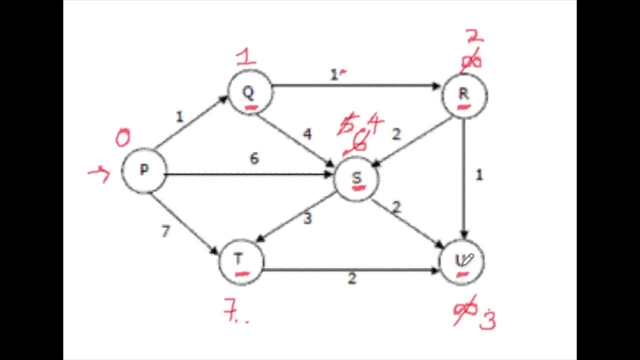 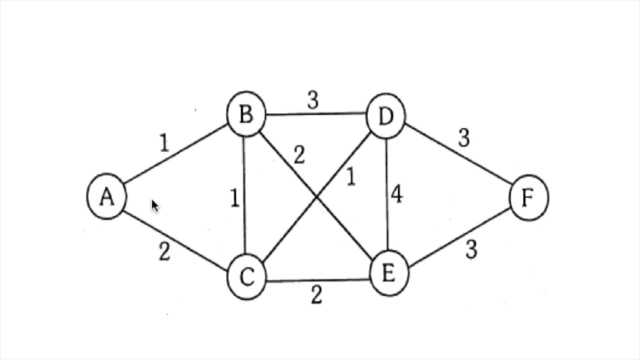 P to U is 3, that is coming via Q and R, and from P to S, it is 4, it is coming via P, Q, R and then S, and from P to T, it is 7 and it is a direct edge path. That's it, one more graph, and let us find out the shortest path to all the vertices using: 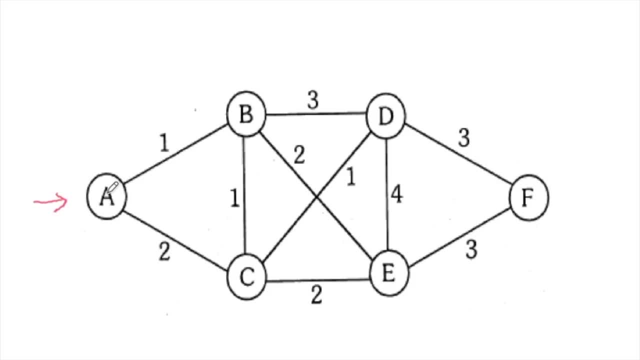 Dijkstra algorithm and this is my starting vertex. I am labeling it as starting vertex, so this is 0, this is 1, 2. no direct edge path. no direct edge path, so it is infinity. now I have to select the shortest word path vertex, that is B. I select this one because it is: 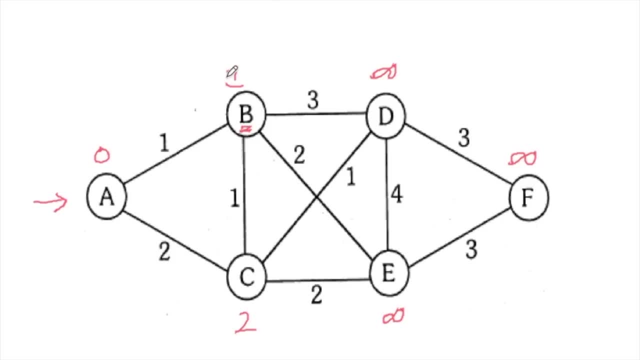 1, 2, infinity, infinity, infinity. so out of all these vertices, this is shortest one which is having distance as 1, so I select this from here. I see, are there any relaxation to any vertex? B to C, there is a edge and 1 plus 1, 2 is already 2, no change. B to D: 1 plus 3, that is 4, so change. 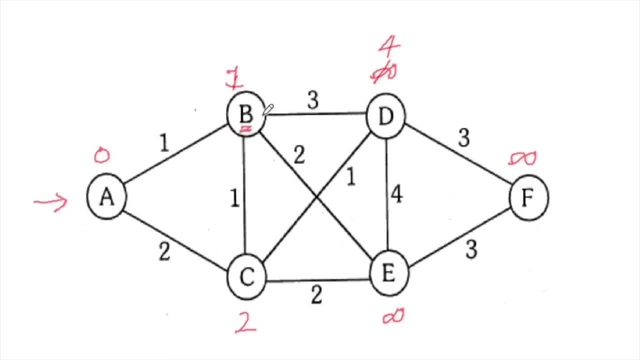 it to 4, B to E, 1 plus 2, that is 3 and it is infinity. change it to 3. that's it. from B. there are 3 edges going out. so this is done. I have relaxed the vertices. now select the next shortest. 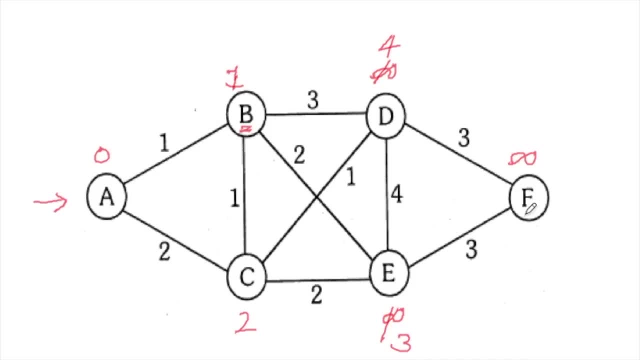 one. So the remaining are C, D, E, F. so shortest one is C. select this one. so it means I have found the shortest path to C. selecting means I have finalized the shortest path from A to C. that cost is 2. now, after finishing this, I see that is there any possibility of changing other vertices: the: 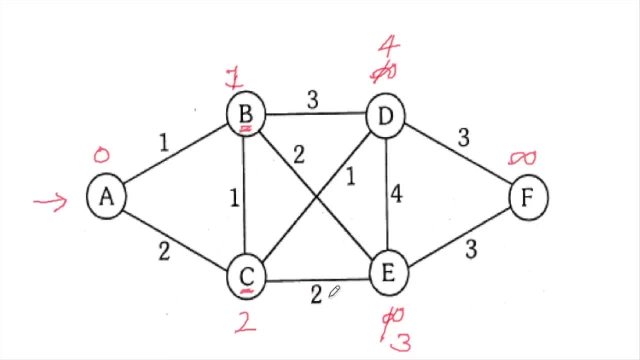 cost of other vertices. so let us see so: 2 plus 2, 4 and it is 3.. There is no change. 2 plus 1 is 3 and this is 4, so change it to 3, that's all. there are only two edges going out from here, so this is updated finished. now I have to select the 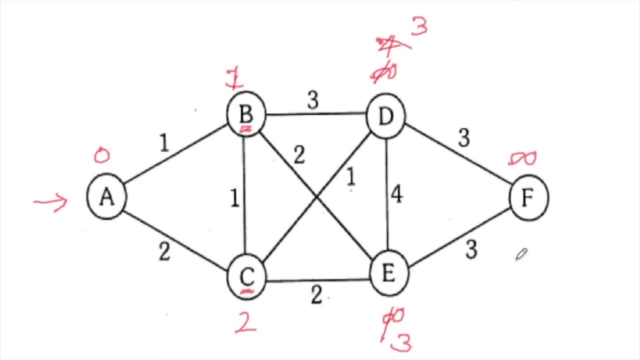 shortest path from remaining, that is, a, D, E and F. these three are remaining. I have not found the shortest path to them, so I will select the minimum one. so D and E- they are of same value, so I select D first. C, D, This is 3 and this is the shortest path to D. so from here I will see. is there any relaxation? 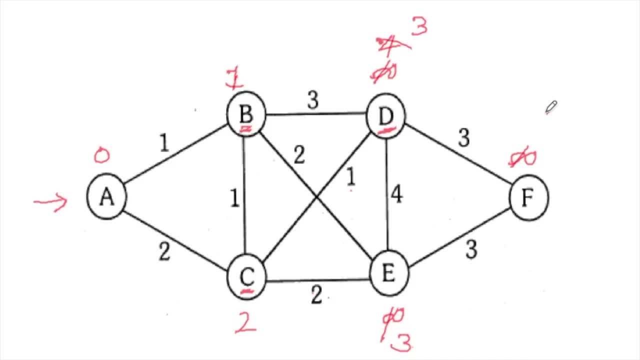 3 plus 3 is 6, so this infinity change it to 6, then 3 plus 4 is 7 and this is already 3, so there is no change. that's all now remaining. two vertices are there: E and F. E is the shortest. 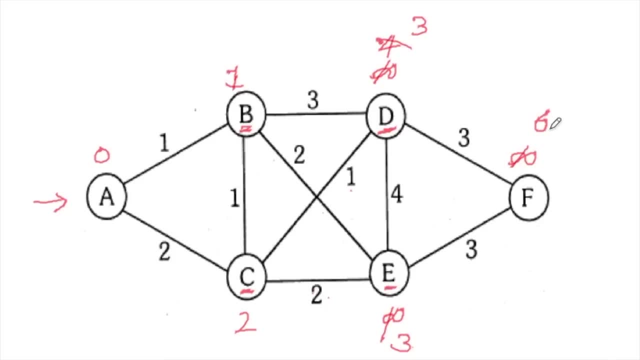 one, so I select this. 3 plus 3 is 6. it is already 6, there is no update, And last vertex remaining is F, so I have selected all the vertices. selected means I have found the shortest path to them and the shortest path starting from A to all other. 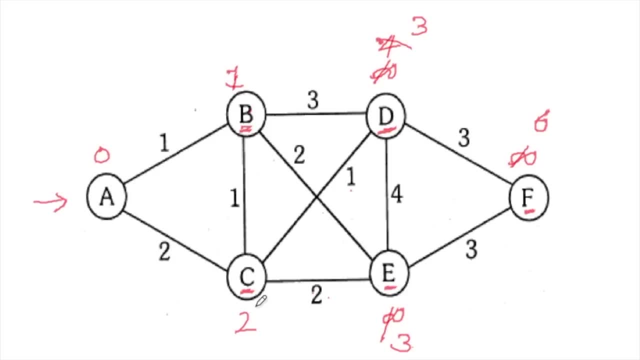 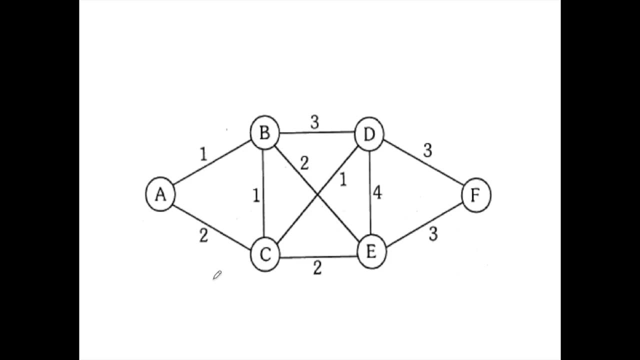 vertices is labeled above those vertices, that is, B is 1, C is 2, D is 3, E is 3 and F is 6.. If you want to analyze the time complexity of this algorithm, for the extra shortest path algorithm, let us say there are V. number of vertices: 1, 2, 3, 4, 5, 6.. 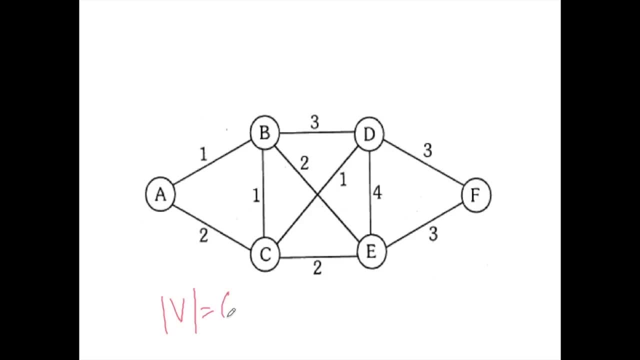 That is, Size of V is 6, so number of vertices are V. so we have to find the shortest path to all these vertices, for from A to every other vertex. so let us say it is V. then while finding shortest path to each vertex, we check: are the other vertices getting relaxed. so how many vertices? 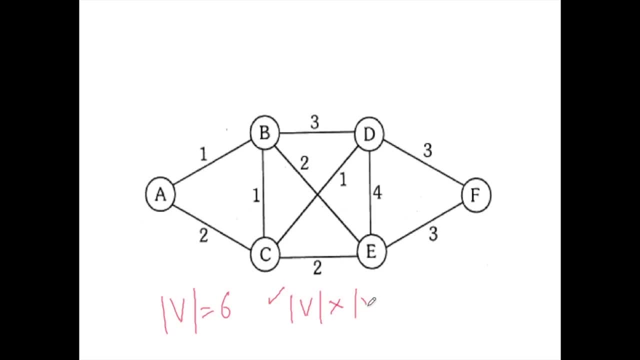 we have to check. at most we have to check V number of vertices every time. let us assume this. So the time complexity will be V square. so if we say there are N vertices, then it will be N square. so it is order of N square, right by using red black tree. it is said that the 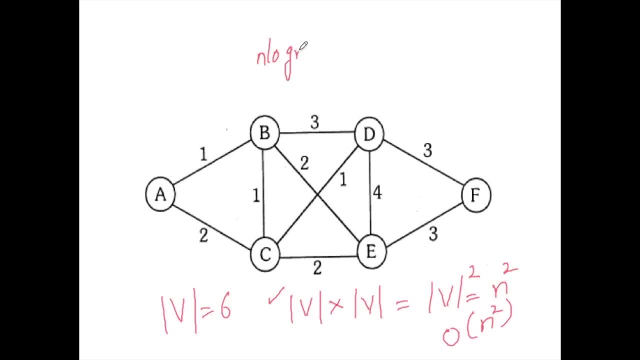 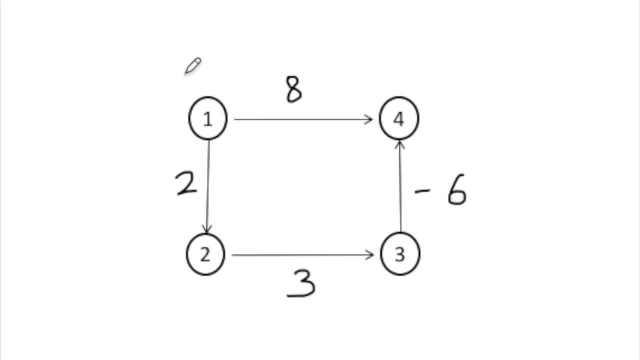 time. complexity of this algorithm will be N, log N and how it will be using red black tree and how it will get this time you can browse through and find out. ok, next we move ahead. What will happen if there are negative edges in a graph? what the extra algorithm will do. 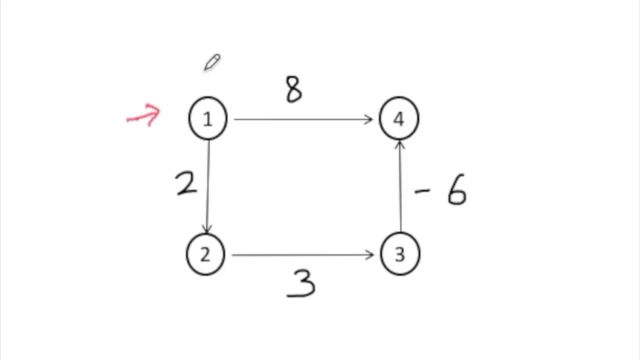 so let me select this as a starting vertex. so this is 0 and this is 8: 2, this is infinity. let us start. I will find the shortest path to this vertex because this is minimum 2, so I will select this vertex first. I will select this vertex. 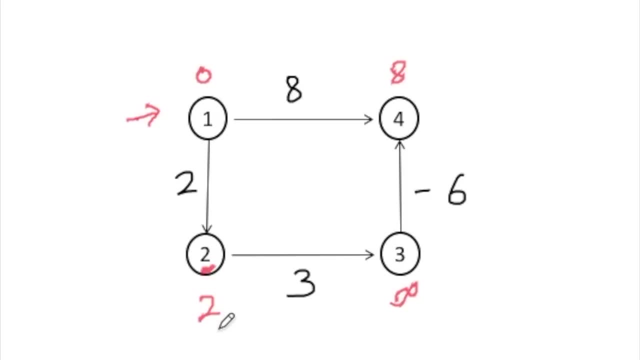 So this is 2. now from here, I check. is there any shorter path to any other vertex? yes, 2 to 3, so this is 5 and it is infinity. I will modify it to 5. that's all. now remaining vertices are 4 and 3 out of this. this is 8 and this is 5, so I will select 5. I will select this. 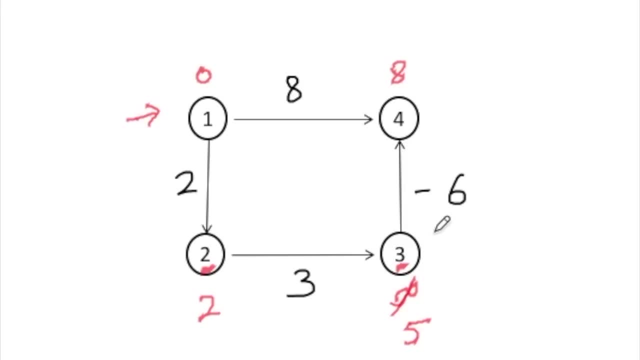 vertex. now let us see: is there any shortest path from here? Ok, 5 minus 6 is minus 1, so this is 8. change it to minus 1 now. the remaining vertex is 4, so I select this vertex and its path is minus 1. that's it. so if there is negative, 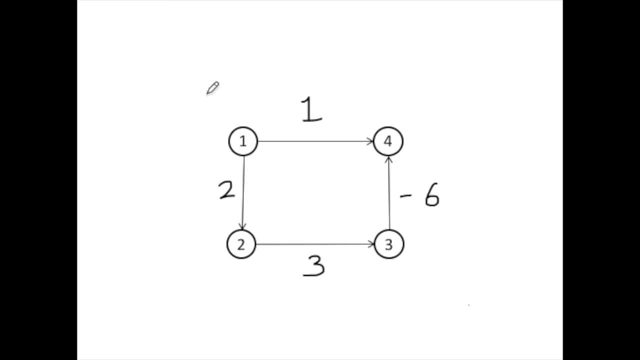 edge. it is working perfectly. let us see what will happen in this graph. I will use the extra algorithm to find the shortest path to all the vertices. this is my starting vertex. so the distance is 0, distance is 1 and this is 2, and there is no direct edge from 1 to 3. 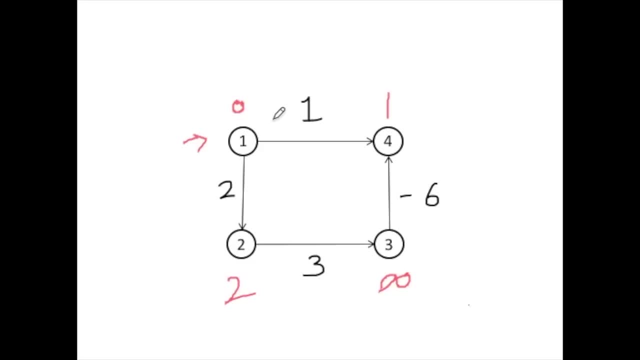 so this is infinity. Now I will start selecting the vertices to find the shortest path. so the shortest one from 1 to infinity is 1, so I select this one. so this vertex is selected. so it means I have found the shortest path. from 1 to 4 is 1. it is finished. 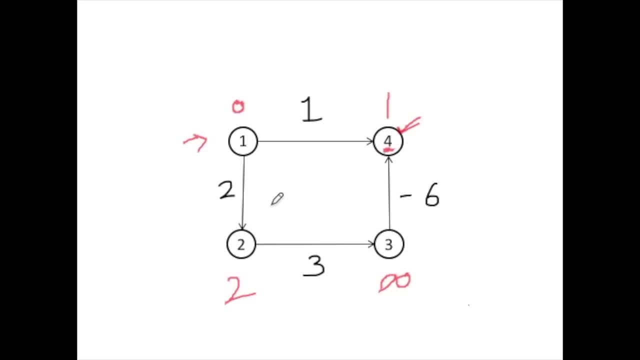 Now I select From here. there are no edges going out, so I select the next one. the next smallest one is 2 and the shortest path is 2, and from here I see that this can be relaxed, so I will change it to 5.. 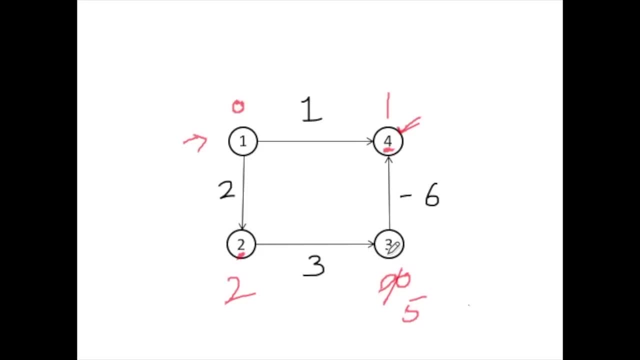 The next one remaining is this one, so I will select this. and once I select this, I will see that will the other vertices get relaxed. so 5 minus 6 is minus 1, so this will change to minus 1.. So here the extra goes wrong. the vertex which I already selected and said that the shortest 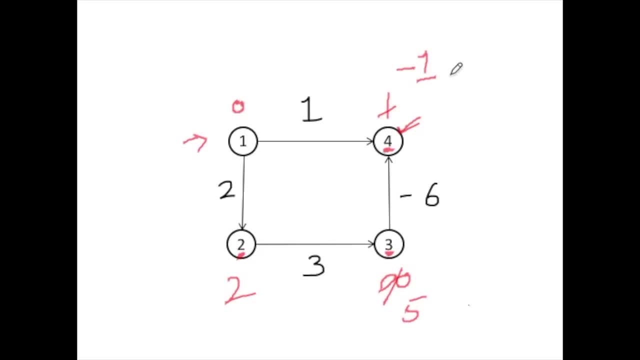 path to this vertex is 1. later its distance is getting modified, its path is getting modified. so it means in the first stage the extra has given me wrong result and as per the extra, the vertices which are already selected, which you have already found the shortest path you. 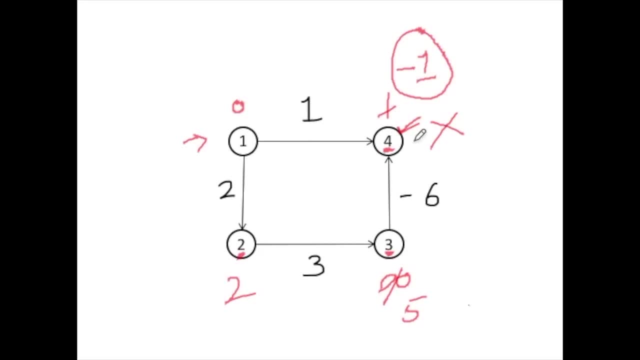 should not relax them. You should not update them, as per the extra algorithm. So what if I try to relax it? it is getting changed. So because the extra says that once the vertex is selected, and that is the only shortest path to that vertex, we don't have to update it further. and it will not get updated at. 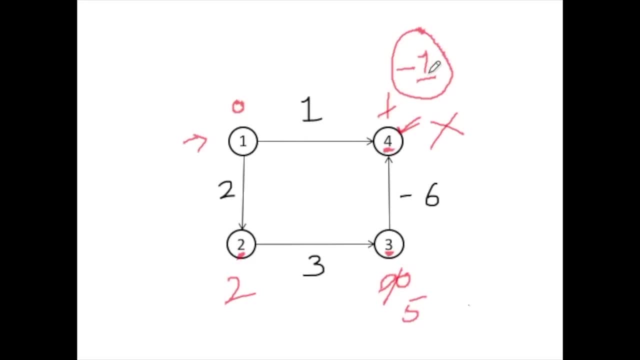 all, but in case of negative edges it is getting updated, it is getting modified, So the extra algorithm may not work perfectly always in case of negative edges. In the previous example where you saw there was a negative edge, this was negative edge and here it was working, and in the other other one it's not working. 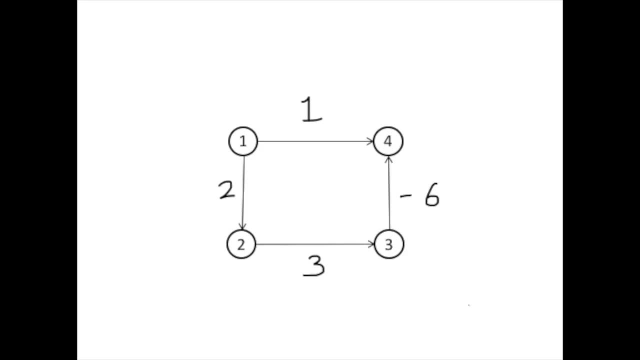 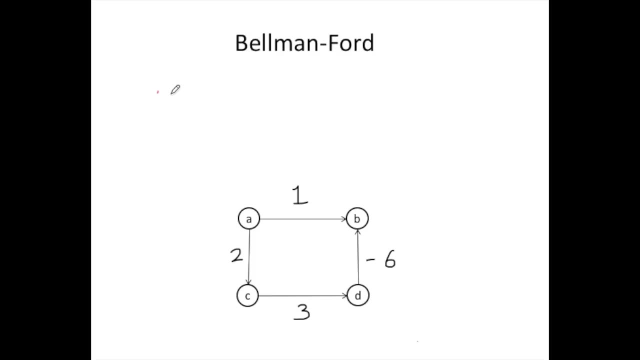 So it may or may not work when there are negative edges. Another algorithm, that is Bellman-Fords algorithm. this algorithm is for finding the shortest path. just now we saw that Dijkstra algorithm was unable to find the path perfectly always if there are negative edges. 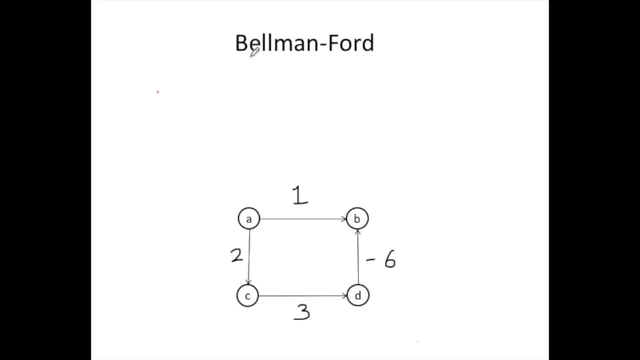 So it may work. it may not work perfectly. So here we have another algorithm which works always when there are negative edges, but though it is also having its drawback. So first let us see it can find out the shortest path in this case. So what? Bellman-Fords says that, in contrast to Dijkstra, where Dijkstra was saying that 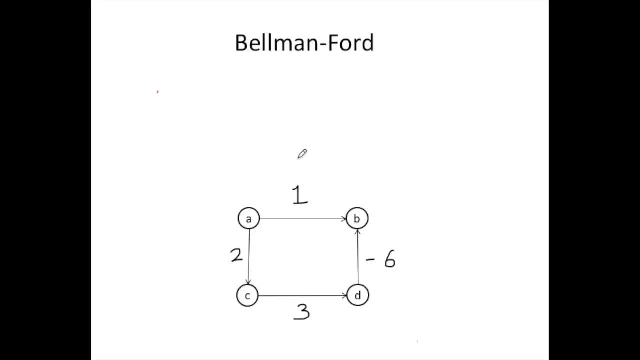 relax the vertices only once. but Bellman-Fords says that go on relaxing the vertices for some number of times so that finally you get the perfect shortest path, Or correct, shortest path to all the vertices. So let us see what he says. I am going to show you the procedure of Bellman-Fords. 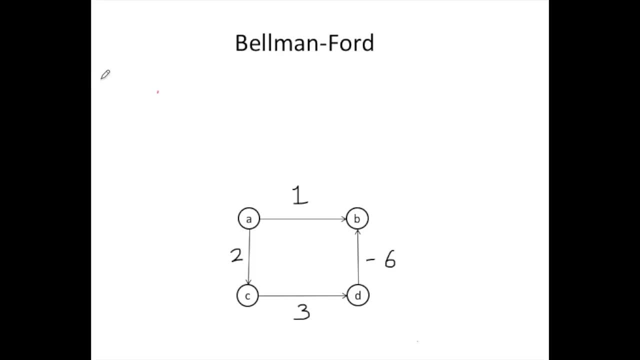 So he says that from the graph you make the list of edges. So here I pick up the list of edges. so I will pick up D to B, the last one. I am selecting this one first, Next is C to D and next is A to C. the next one is A to B. right, these are the list of. 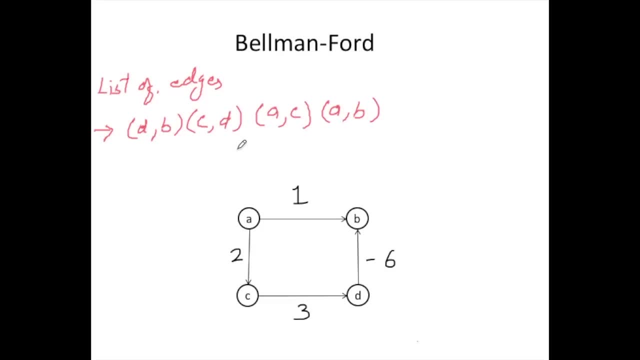 edges. So I have only four edges. I have taken a very simple graph to understand this. So I have not started from A to B, I have started from D to B. you can realize why I did so. So let us follow the procedure, What Bellman-Fords says. first step is take the list of all edges and mark the distances. 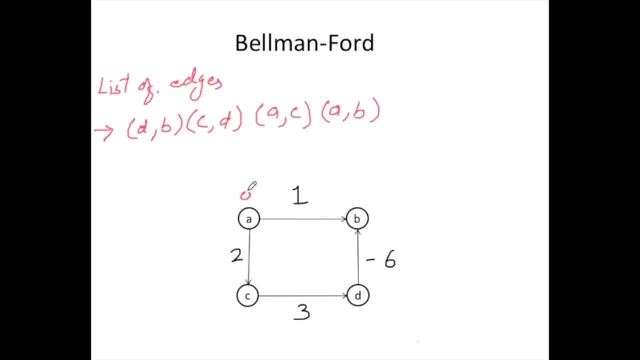 for all the vertices. so this is zero and make all these as infinity. even there is a direct edge path available, but do not consider it, mark it as infinity only. So the starting vertex, that is the source vertex, mark it as zero. rest of the vertices as infinity. 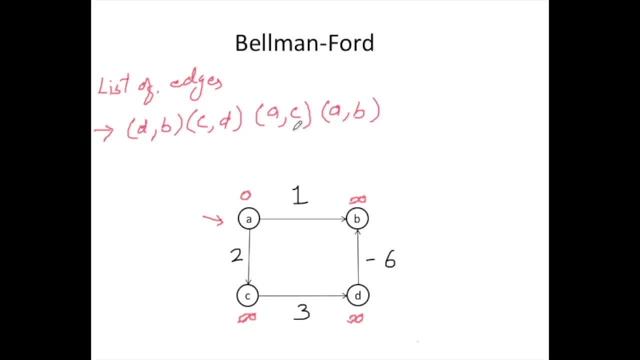 That's it now. go on relaxing the edges. for how many times? number of vertices are four, so do it for number of vertices minus one times, that is three times. go on relaxing them. Let us do it. D to B, D is infinity. so infinity minus six is infinity only, and this is all. 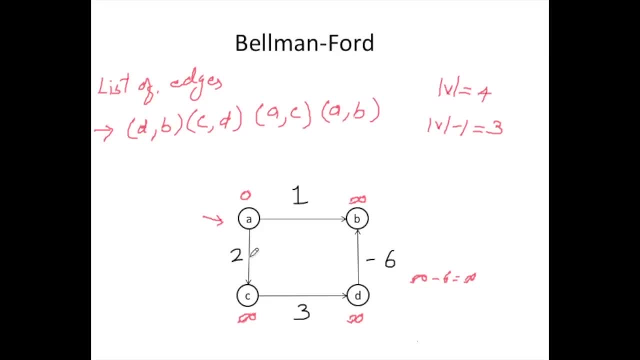 already infinity, so there is no change. then C to D: infinity plus three is infinity only, and this is not less than infinity, so this is infinity only. A to C. A to C. zero plus two, zero plus two, this is zero and two. zero plus two is two, this is infinity. so change it to. 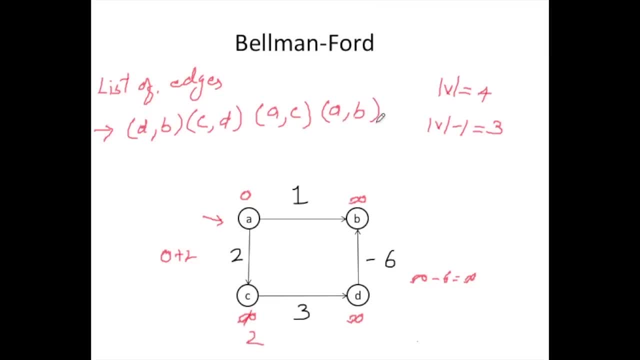 two. two is smaller than infinity. Then A to B: zero plus one, one, So this is infinity. one is a smaller than infinity. change it to one, so this. I have done it one time, so I will maintain the count, so I have finished it for one time. 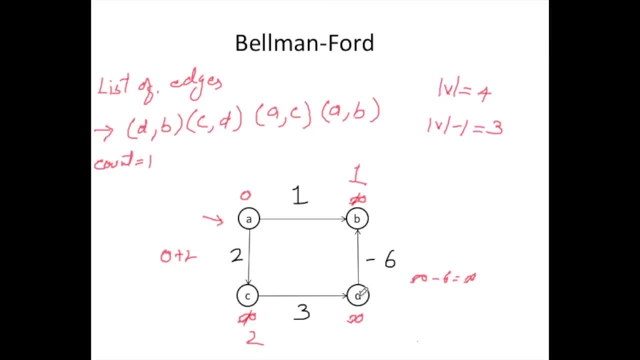 Now let me repeat once more: D to B: D is infinity to B, infinity minus six is infinity, and that is one, so it will not change. C to D: two plus three is five, right, so this will change to five. Then A to C: zero plus two is two, and it is already two. A to B: zero plus one and one it. 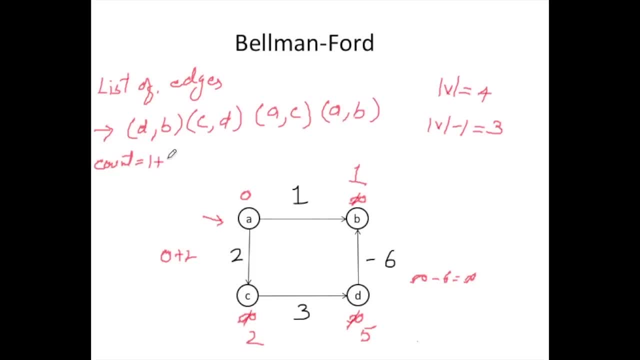 is already one. so I have done it for two times. so one plus one, two times. now let me repeat one more time: D to B: five minus six is minus one, and this is already one. change it to minus one. Then C to D: two plus three is five, it is already five. 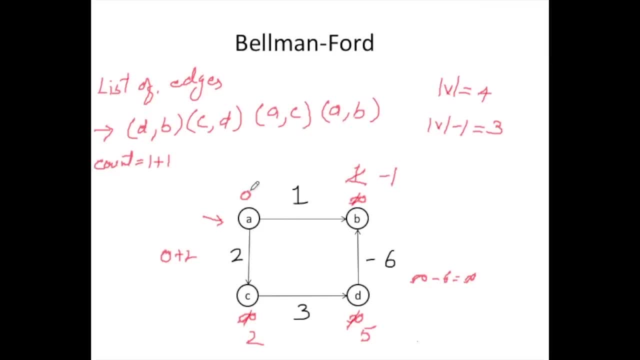 A to C: two plus three is five. A to C: zero plus two is already two. A to B: zero plus one and one. this is minus one, so one is not less than minus one, so no change. So that's it. I have finished it for third time. 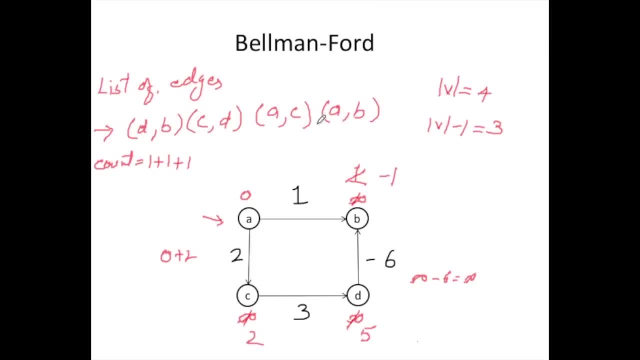 So I have completed the relaxation of all the list of edges Three times. because there are four vertices, I have to do it for three times. So the idea behind Bellman for this: go on repeatedly relaxing the vertices for Three times, v minus 1 times, and all the vertices will definitely get relaxed and finally you get. 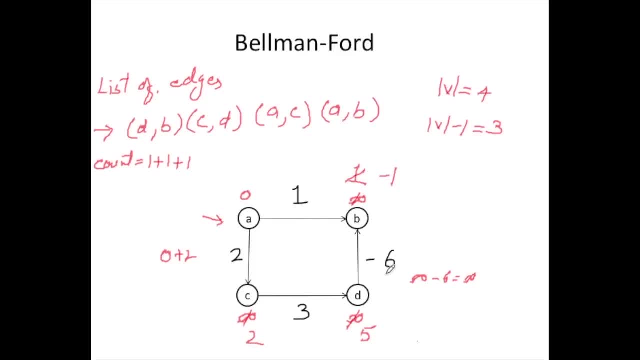 the correct, shortest path to all the vertices, even in case of negative edges. right? How much time Bellman-Ford algorithm takes, as there are e number of edges and we have to go through all of them. for how many times? v minus 1 times. v minus 1 times. so this is e into v. v is n, so this is. 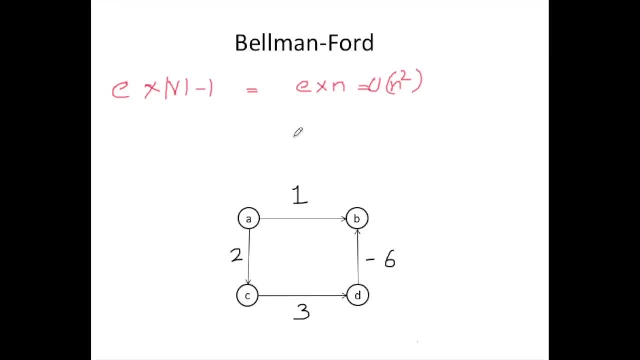 almost n square right. v is there. just we are relaxing all that just one by one. so e number of edges and how many times we are doing it. number of vertices minus 1. number of vertices. let us say n. so e into n. so if you say both are. 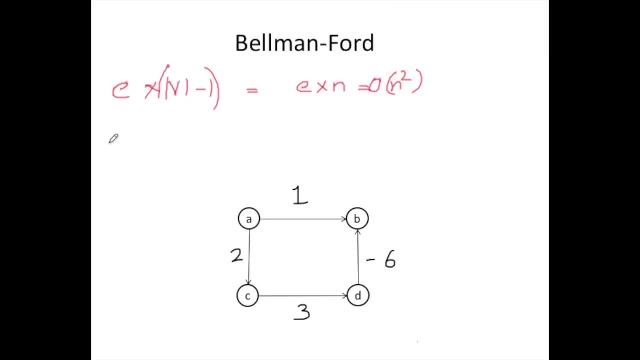 n, n. so it is order of n square. and sometime, if there is a complete graph, let us say the graph is like this: if there is a complete graph, in a complete graph, you know that the number of edges will be equal to n into n minus 1 by 2, so this will be n square edges. so then the time complexity. 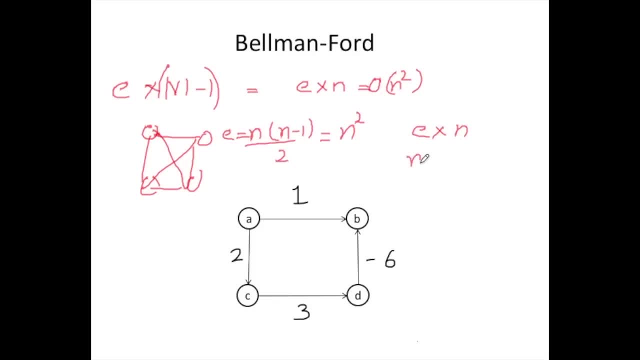 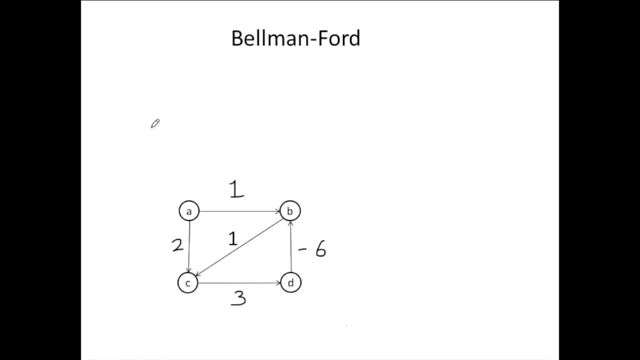 will be e into n and e itself is n square. so n square into n will be n cube. so the time complexity of bellman ford, in case of complete graph, in case of complete graph, will be order of n cube. now let us see what will happen in this graph. i have just added one. 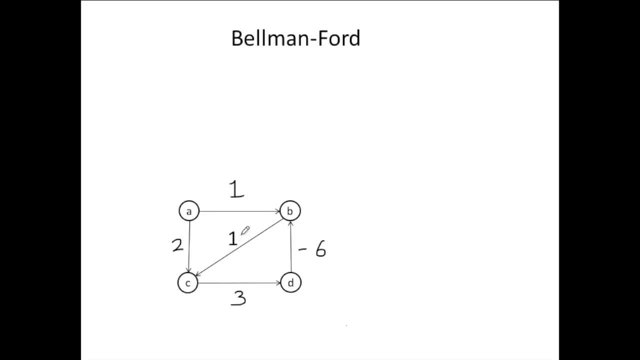 more edge here with the cost as one. so it's just same as previous graph, but just a new edge is added. so i'll perform bellman ford on this one. i'll take the list of edges: d to b and c to d, a to c, a to b and b to c. 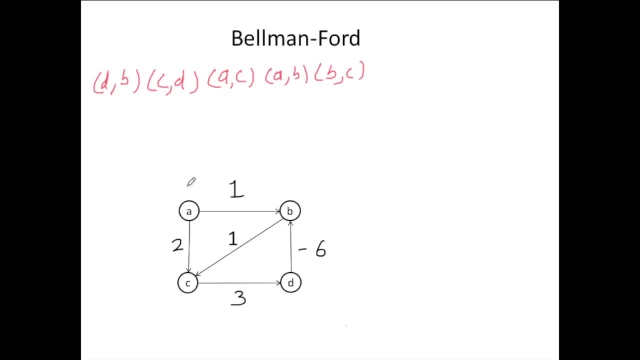 so let me go on relaxing all of them. so first i label the vertices: this is zero and this is infinity. so to all of the vertices we should make it infinite. let us relax: d to b, infinity minus six. infinity- no change. c to d. c to d, infinity plus three. infinity- no change. a, c, zero plus two. 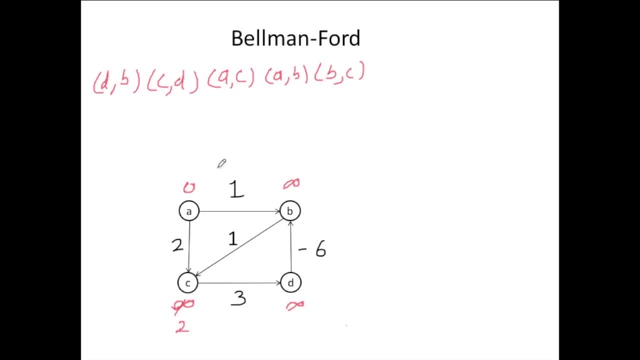 that is infinity here, so it will change. this is smaller: a to b: 0 plus 1: 1, so this will change to 1. then b to c: 1 plus 1 is 2 and it's already 2. no change. now relax again. d to b: infinity minus 6: there is no change. 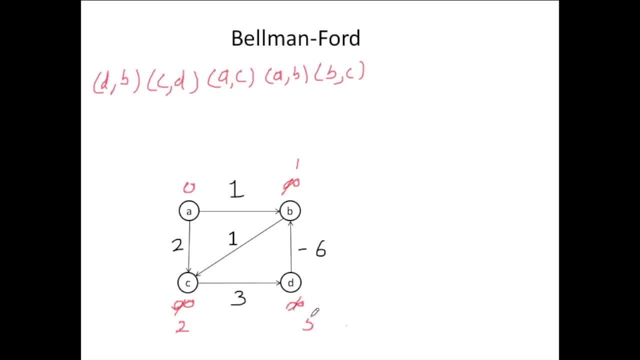 c to d: 2 plus 3, 5, so this will change to 5.. a to c: no change. a to b: there is no change, and b to c: b is 1, 1 plus 1 is 2, then it will remain 2 only. so i have finished two times so far. in third time. 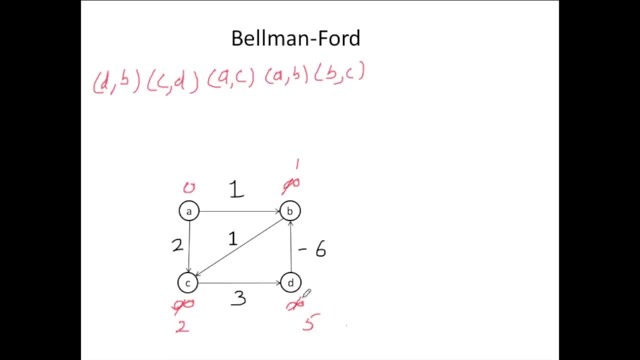 d to b: 5 minus 1. sorry, 5 minus 6 is minus 1, so this will change to minus 1. then c to d: 2 plus 3, 5 as it is a to c: 0 plus 2, that is 2 only a to b, 0 plus 1, and it's already minus. 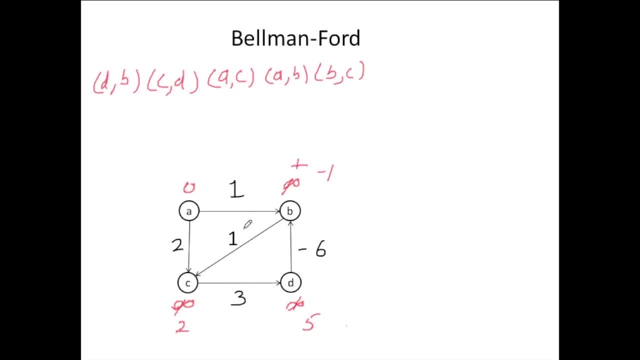 1, which is smaller, so no change. b to c minus 1 and 1. s is 0 and this is 2, so this will change to 0.. i have finished for three times, but i relax one more time and see what will happen as bellman. 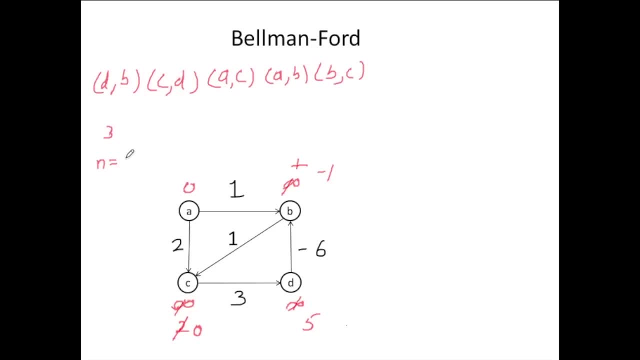 was saying that if there are three, four vertices, you relax all of them for three times, every vertex will have a shortest path and it will be a correct shortest path. that's what bellman ford was saying. let us try it again once more. let us relax all of them. d to b. 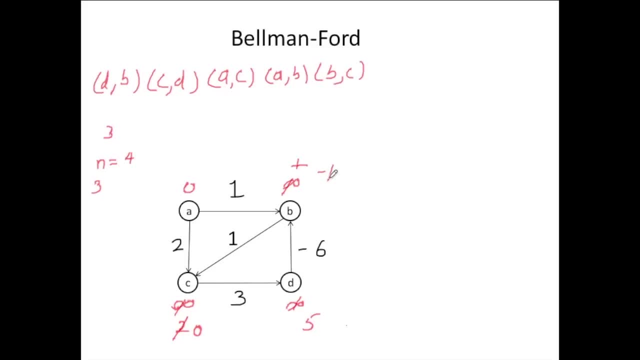 5 minus 6 is minus 1. only right then c to d, c to d: 0 plus 3 is 3 and it is not 5. so change it to 3. 3, 5 was greater, so 3 is smaller. a to c: a to c: 0 plus 2, 2, only a to b, it is 1. it's minus 1 already. 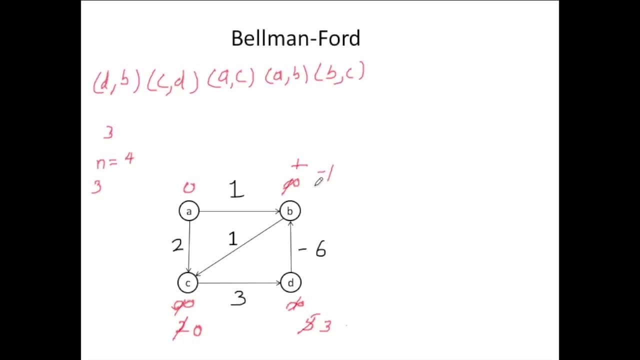 is better. then b to c, it's minus 1 and 1, that is 0, no change. so you can see that after finishing it for three times, i got one of the vertex relaxed. that was 5 and it became 3. so there is a change. 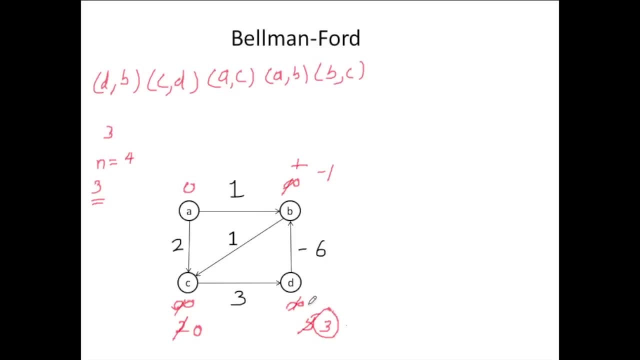 if i repeat once again, definitely i'll find some more vertices. get relaxed, let me do it again: b to d, sorry, d to b. so 3 minus 6 is minus 3, so this will be: minus 3 minus 3 is smaller than minus 1. c to d. 0 plus 3 is 3, that's as it is: a to c. 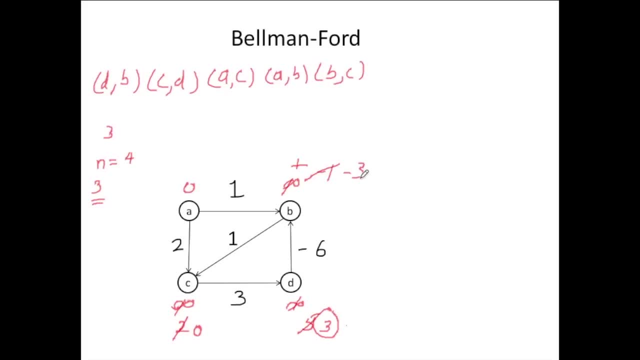 that is as it is a to b, as it is b to c minus 3, and 1 is minus 2. it's also getting relaxed. two vertices are getting so it means, if i go on checking the condition, all these list of vertices, the vertices may be changing their distances again and again. so what's the problem here with?